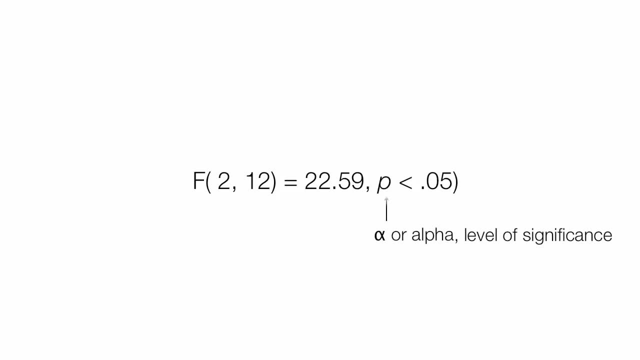 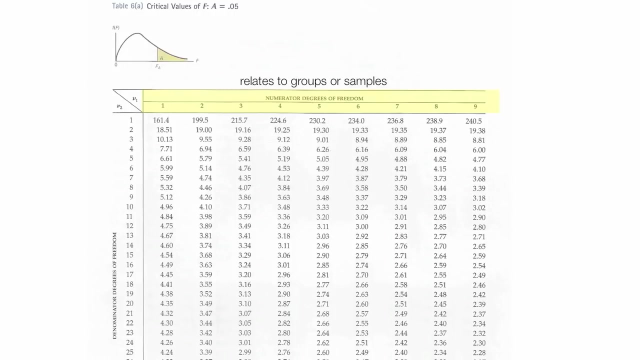 And finally, this P is alpha And it represents the level of significance, in this case .05.. Now, across the top of all these tables, is the degrees of freedom of the numerator, and it relates to the groups or samples. Along the vertical axis is the degrees of freedom of the denominator, and it relates to the number of observations. 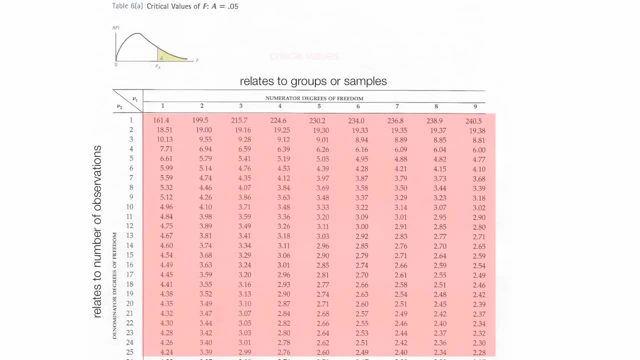 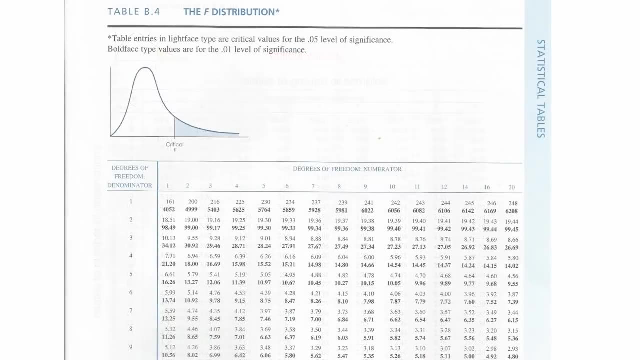 And in the body of the table are critical values, all your critical values. Often you'll see tables like this, And across the top are degrees of freedom for the numerator and on the vertical side are degrees of freedom for the denominator. Notice it has a level of significance of .05, which is that .05 there. 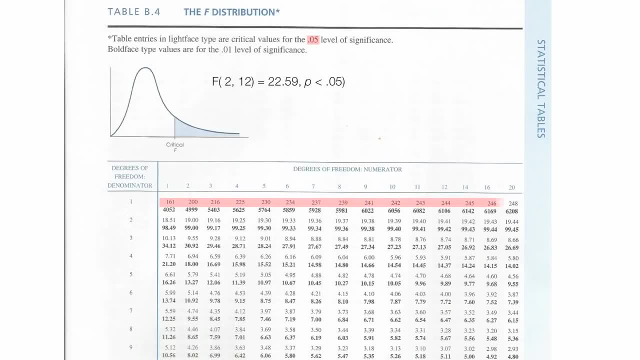 And I'm going to highlight all the red and red dots, And I'm going to highlight all the red and red dots, And I'm going to highlight all the red and red, all the critical values for .05.. Now also, the table has critical values for .01.. 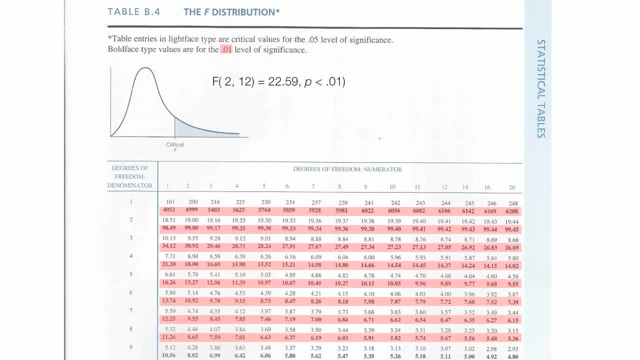 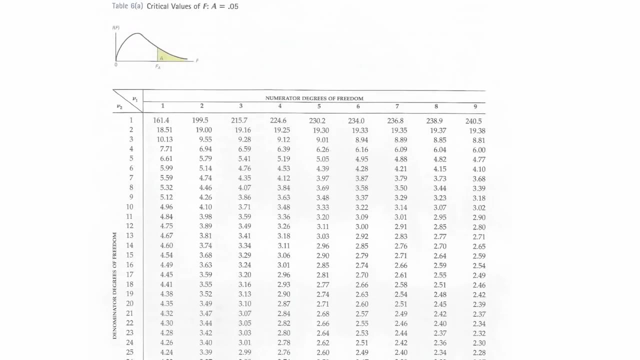 And that's all the bold values in the table. So you have both .05 and .01 critical values. So it's kind of confusing, to say the least. Now I'm going to look up a very specific critical value. Now I'm going to look up a very specific critical value. 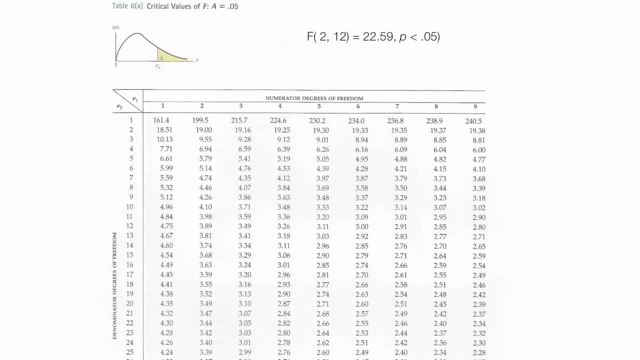 And show you how to do that. And again, the level of significance is .05.. And I'll just check that. And that's what that A is equal to. .05 means alpha or level of significance, And that's what that A is equal to. .05 means alpha or level of significance. 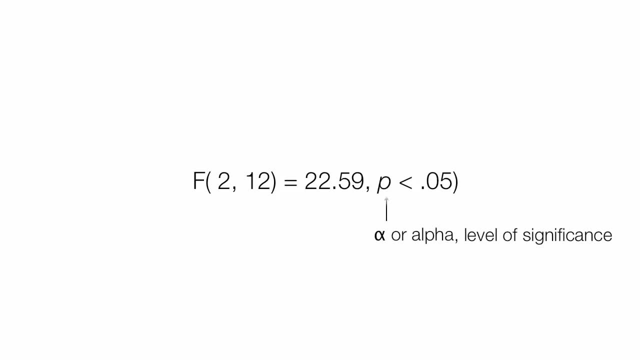 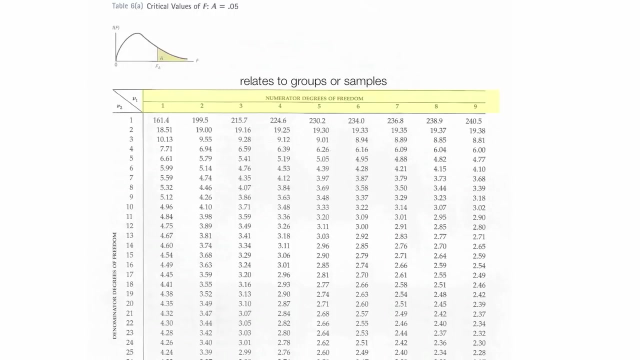 And finally, this P is alpha And it represents a level of significance, in this case 0.05.. Now, across the top of all these tables is the degrees of freedom of the numerator, and it relates to the groups or samples. Along the vertical axis is the degrees of freedom of the denominator, and it relates to the number of observations. 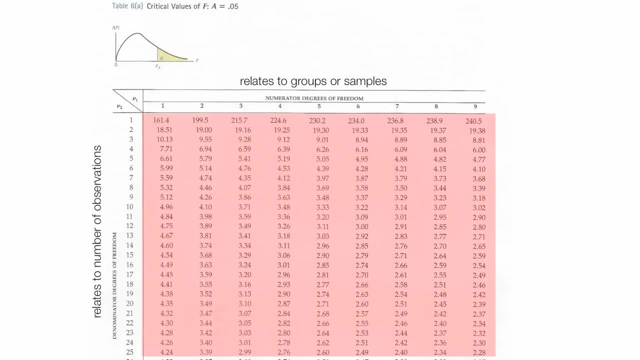 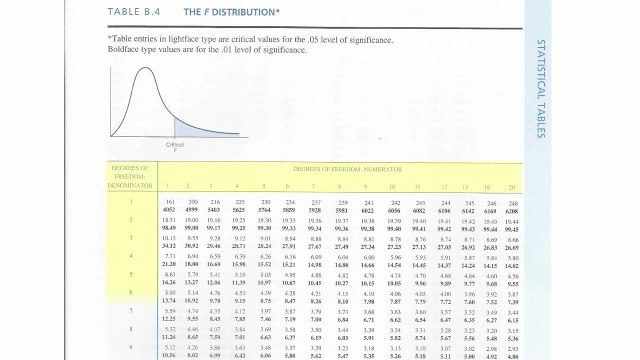 and in the body of the table are critical values, all your critical values. often you'll see tables like this, and across the top are degrees of freedom for the numerator and on the vertical side of degrees of freedom for the denominator. notice it has a level. 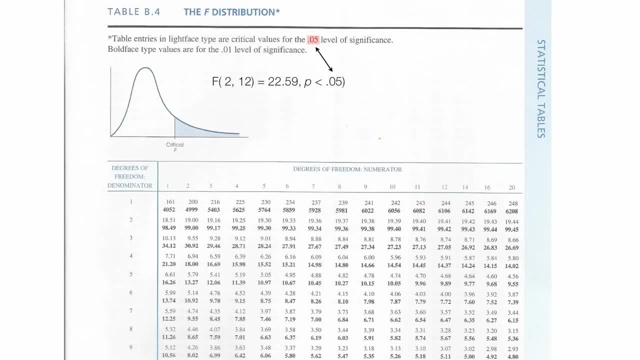 of significance of 0.05, which is that 0.05 there and i'm going to highlight all the red and red, all the critical values for 0.05. now also, the table has critical values for 0.01. and that's all the bold values in the table. 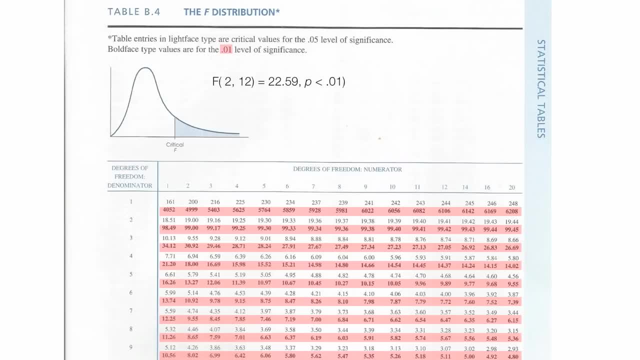 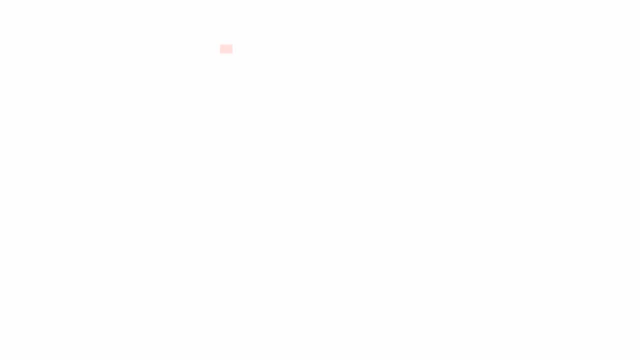 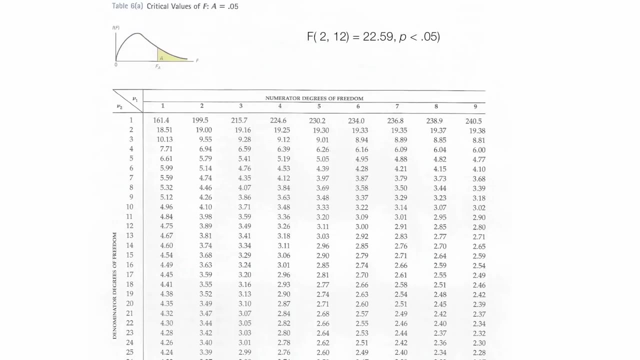 so you have both 0.05 and 0.01 critical values, so it's kind of confusing, to say the least. now i'm going to look up a very specific critical value and show you how to do that. and again, the level of significance is 0.05 and i'll just check that and that's what that. 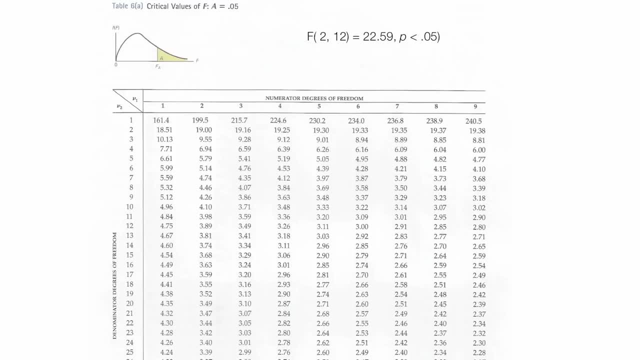 a is equal to 0.05 means alpha or level of significance. the first number is the degrees of freedom of the numerator and that's across the top or the columns, and it's that column right there which is the two column. the second value we look up is the 12 and that's degrees of freedom of the denominator and it's row. 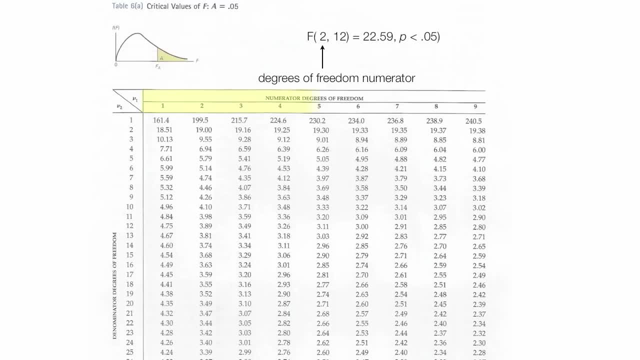 The first number is the degrees of freedom of the numerator And that's across the top or the columns, And it's that column right there which is the 2 column And it's that column right there which is the 2 column. 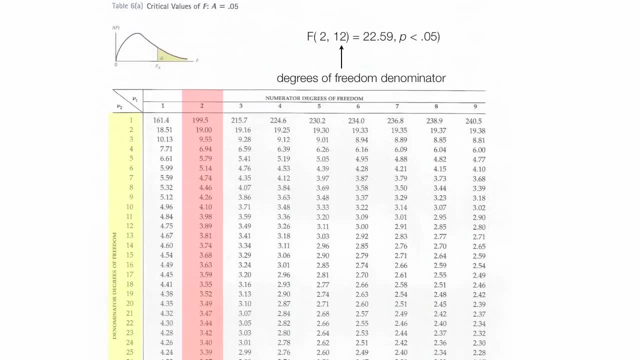 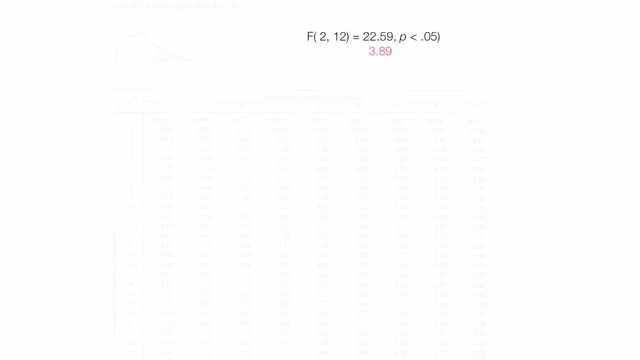 The second value we look up is the 12. And that's degrees of freedom of the denominator And it's row 12. So I'll just fill that in right there. And where they intersect is the critical value, And in this case it's 3.89.. 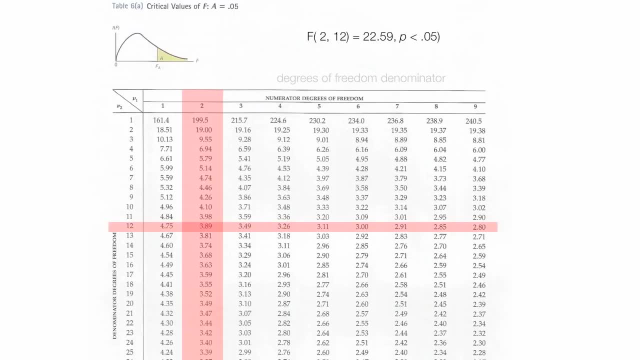 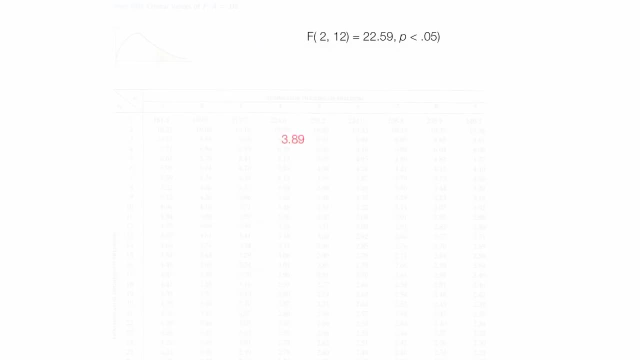 so i'll just fill that in right there. and where they intersect is the critical value, and in this case it's 3.89. so the critical value is 3.89 and i'll draw in my little curve so we can see. i always like to visualize things.